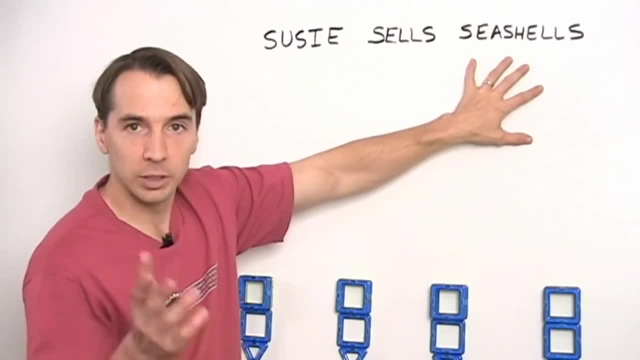 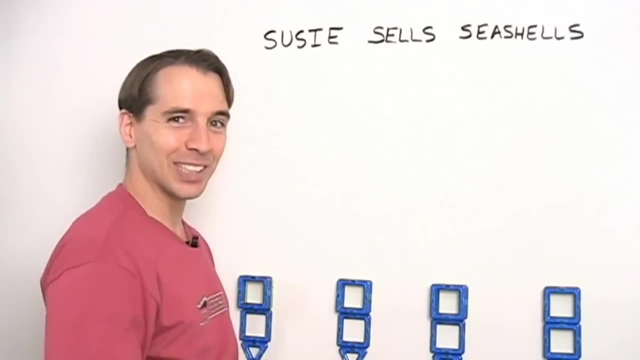 Susie, How many ways can we arrange cells? How many ways can we arrange seashells over here? Before we get into that, you're probably wondering what these are down here. These are magical time saving devices that are going to save you time during this lesson. They're not going to save me. 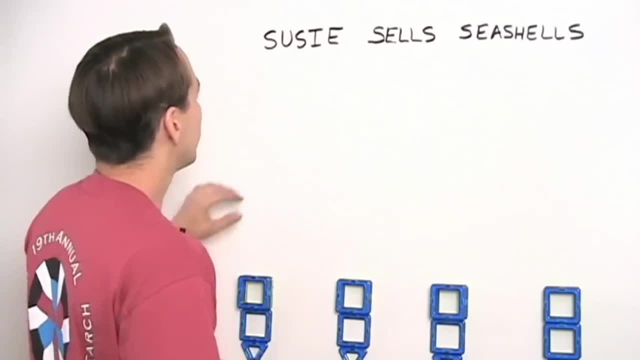 any time. but they're going to save you time And you'll see how in a little bit. We're going to get started with Susie here. Now, if Susie would just be kind enough to spell her name with a Z. 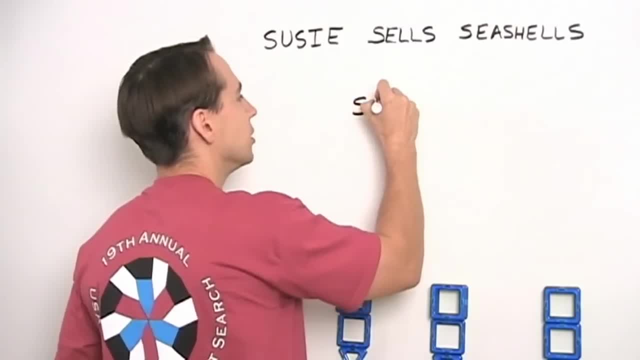 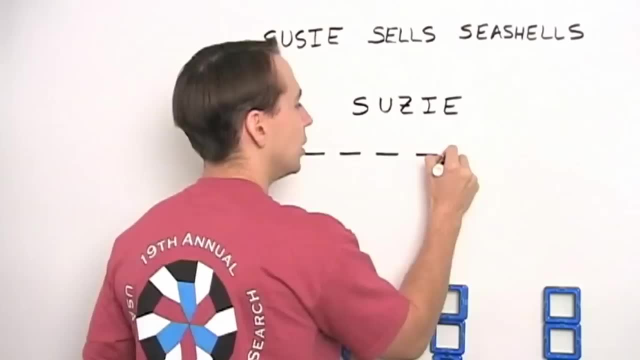 counting the number of ways to arrange these letters would be pretty easy. Let's take a quick look at that Susie with a Z here. well, it's five letters. And to make words out of these five letters, well, we have five choices. for the first letter, Say we pick Z. 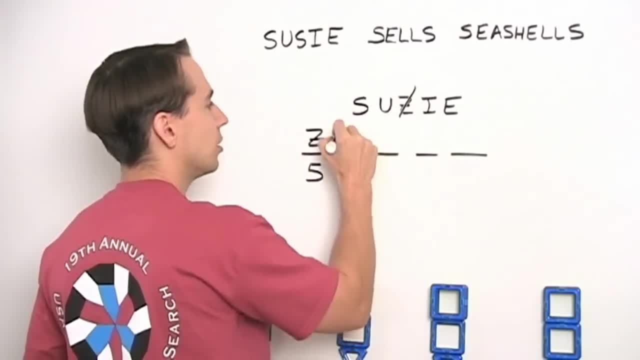 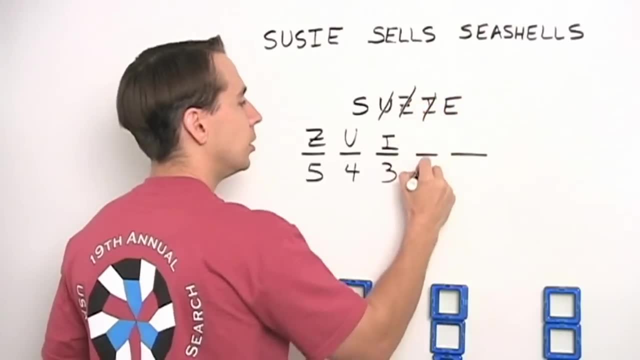 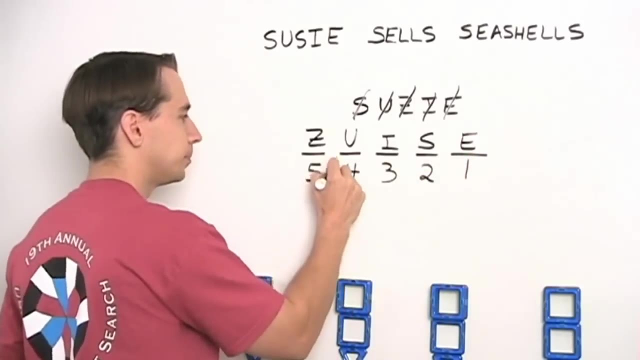 And we have four choices left for the next letter. Say, we pick the U And now we have three choices left for the next letter And two choices left for the next to the last letter. And then we just take the last remaining letter for the final one And we see that there are five factorial words. 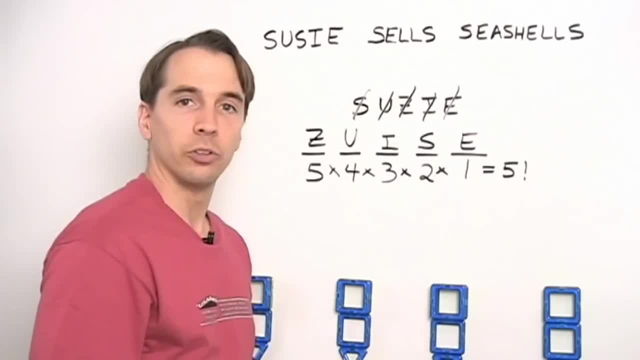 that we can make with the letters in Susie when she's spelling her name with a Z. But of course Susie is not going to be able to spell her name with a Z, But of course Susie is going to be. 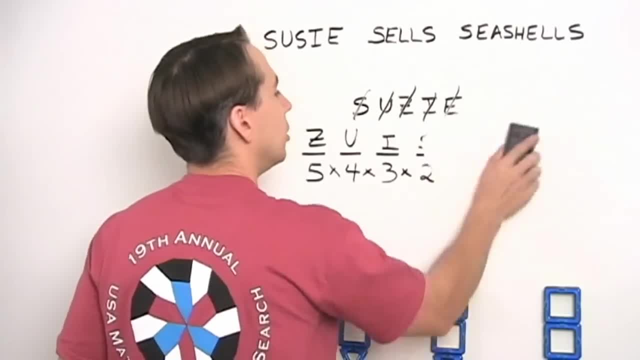 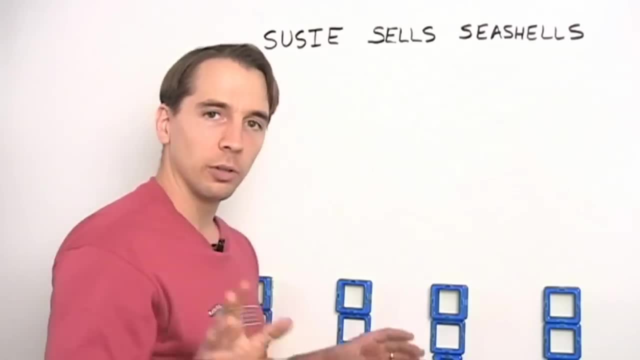 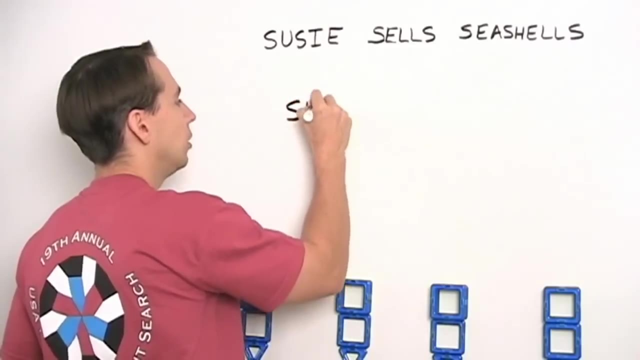 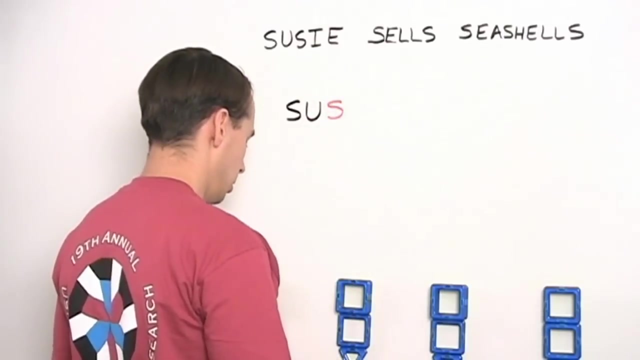 difficult. She insists on using two S's. Let's take a look at why this gives us a little difficulty, And the way we're going to take a look at that is: first, we're going to pretend the two S's are different, And the way we'll do that is we'll color one of them red And we're going to look at 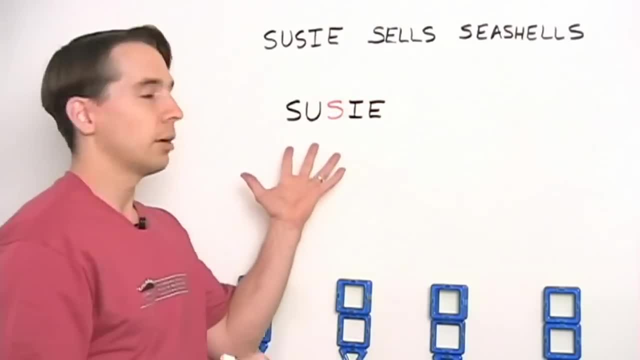 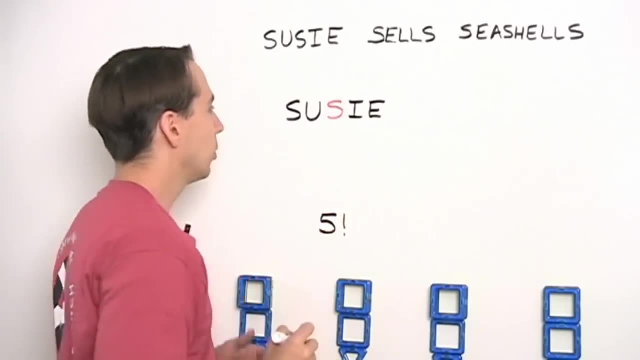 the number of ways to arrange this way. Uh-huh. Now, the two S's are different, So we have five different letters. We already know how many ways we can arrange this. It's five. factorial. This is the same thing as with the Z. Let's take a look. 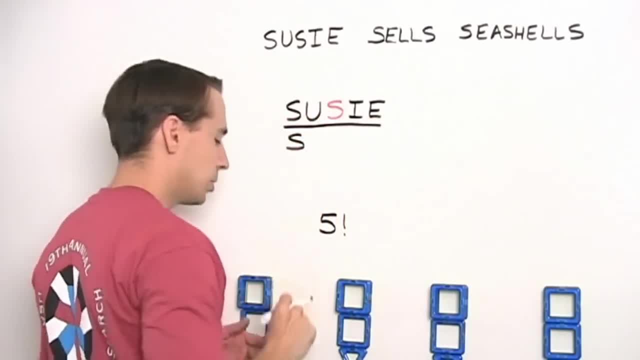 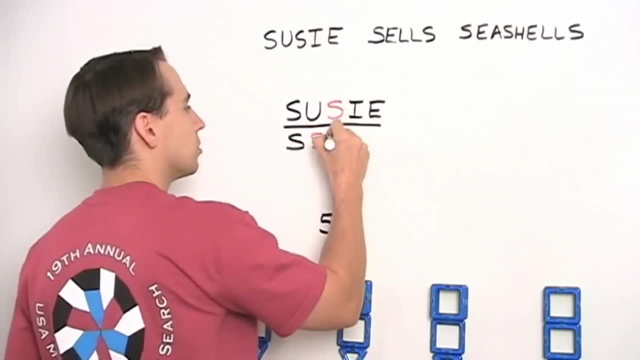 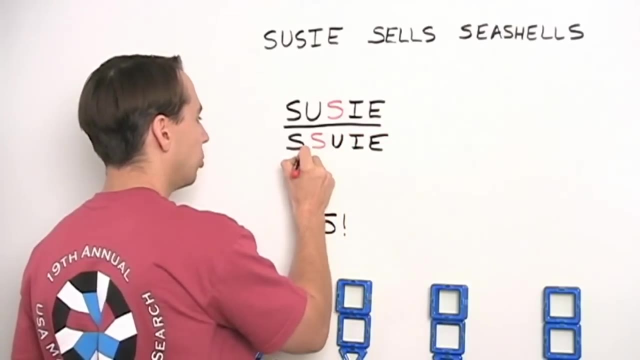 at a couple of these words. So we start with the black S and then use the red S, and then we just write down the rest of the letters. But we also could have started with the red S and then the the black S. So just basically, all we're doing here is switching the two S's. 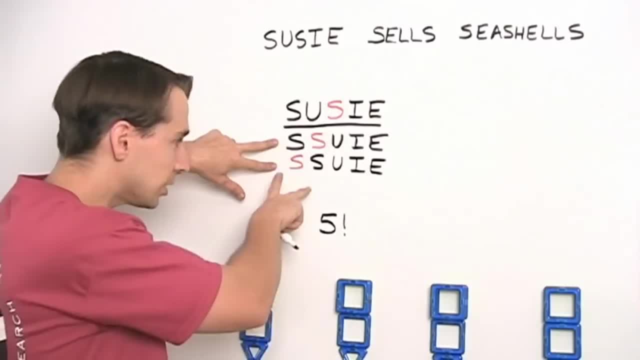 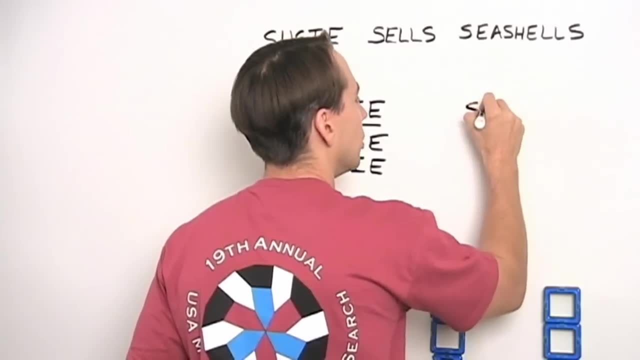 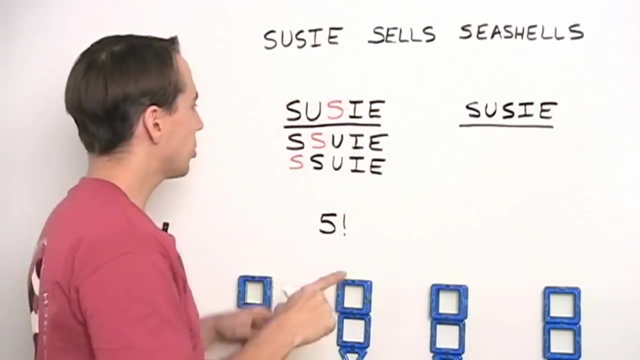 Now when the S's are different. these are two different words. These S's are different, completely different letters. but let's look at what happens when the S's are the same. When our S's are the same, look what happens to these two words. 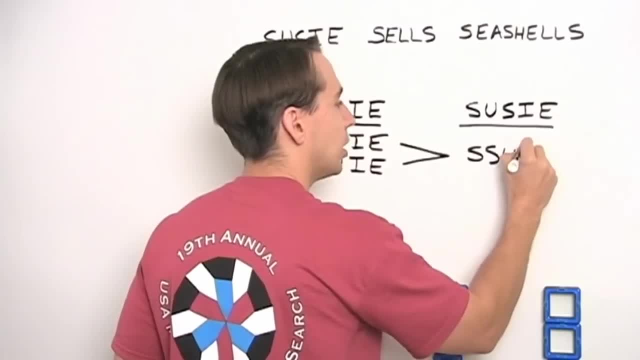 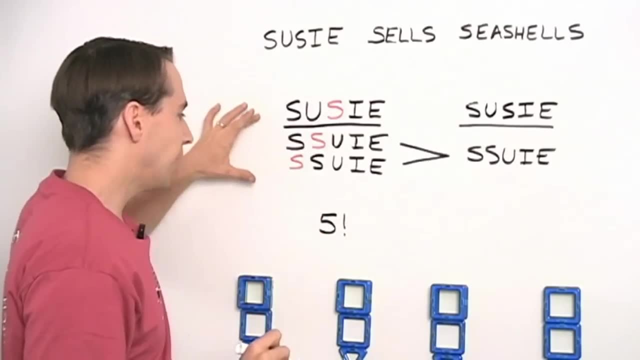 They become the same word. The only difference here is the order of the S's. So when we list out the five factorial words for Susie with the red S, we get 120 words that can be grouped into pairs like this, where the only difference between the two words in each pair is the order of the S's. 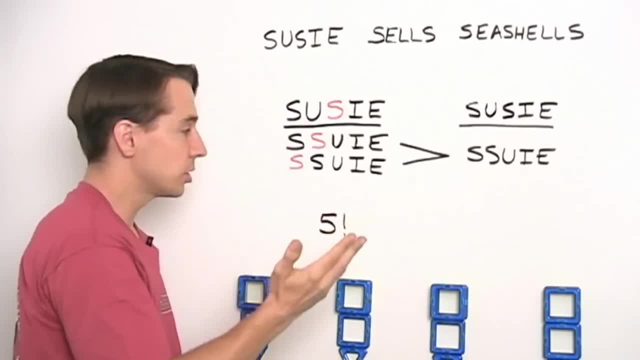 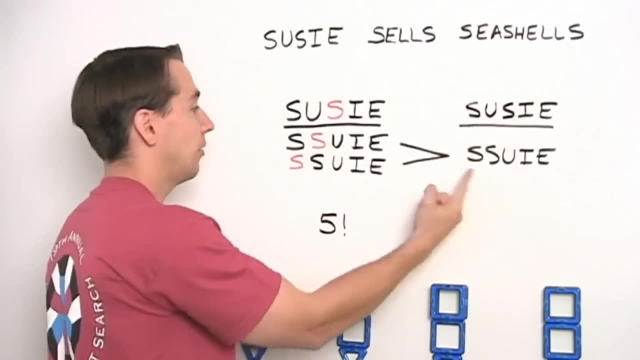 So we of course have five factorial divided by two, which is 60 of the pairs in this list over here. So when we make the list for Susie with the S's the same, we're going to have half as many words as when the S's are different. So in this list 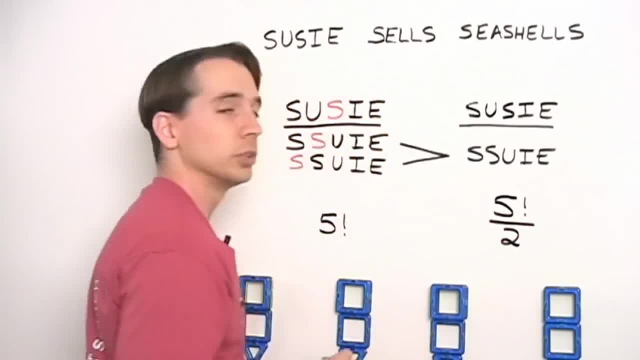 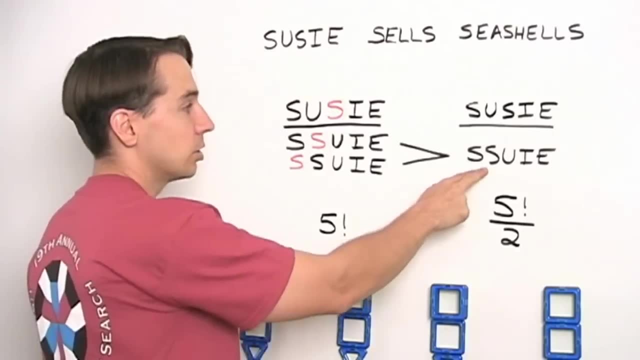 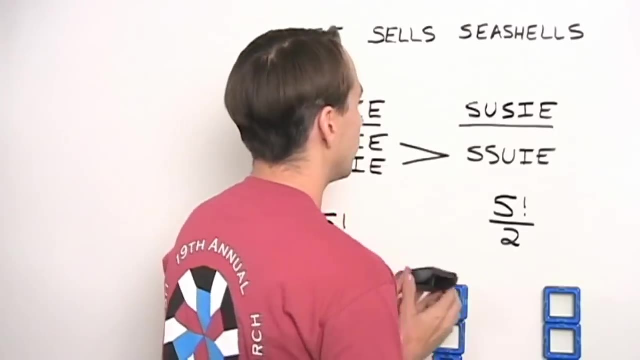 we'll have five factorial divided by two words, Or again we're dividing by two to account for the fact that our S's can come in two different orders. So each of these words will get produced twice. So we've taken care of Susie. She proved not to be so difficult after all. 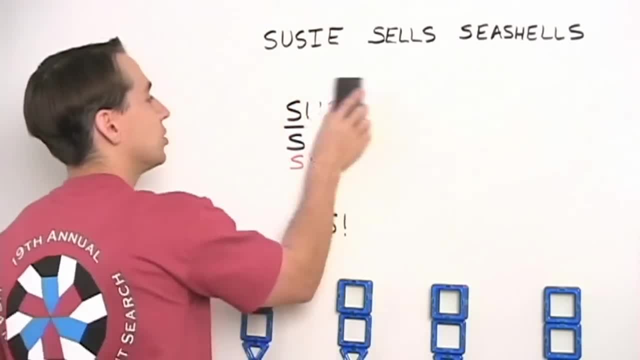 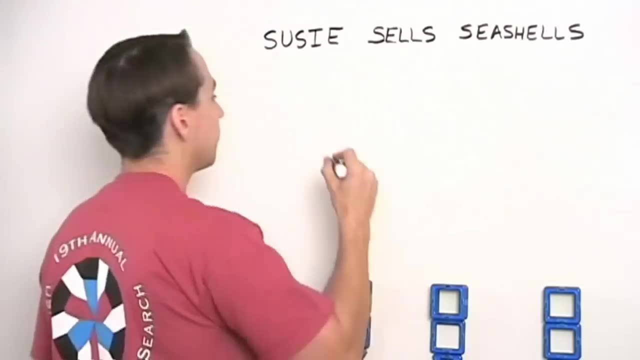 And now we'll move on to cells And we'll get a chance to use our magic time-saving device. First we'll go ahead and write down the answer. for Susie, That was five factorial five letters divided by two for the two S's. 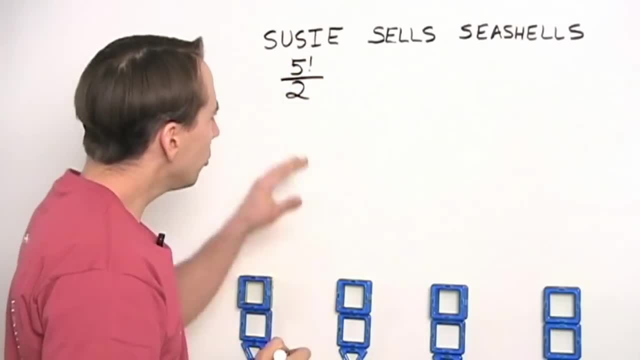 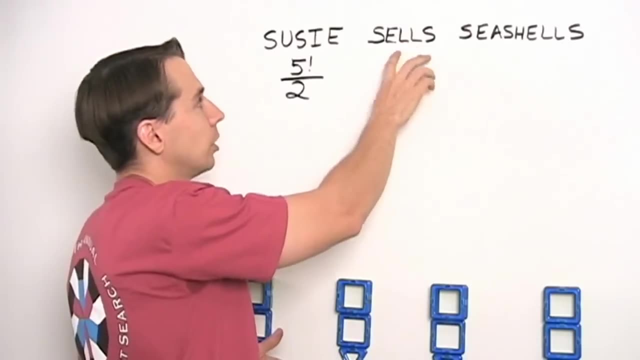 So now we'll look at cells And we're going to do the same thing we did with Susie. We're going to start by thinking about what would happen if the L's were different colored them two different colors and the S's are different colors. 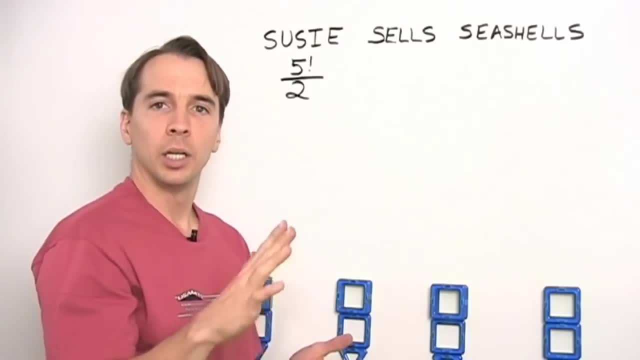 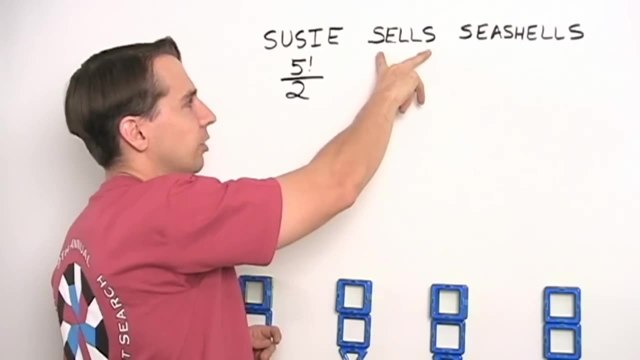 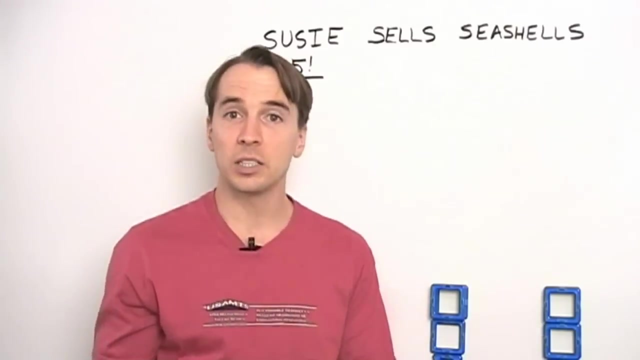 Then all five letters are the same And we'll have five factorial ways to arrange the letters. But then what happens when we make the S's the same and the L's the same? And to get an idea of exactly what happens, what we do is go ahead and make some lists. 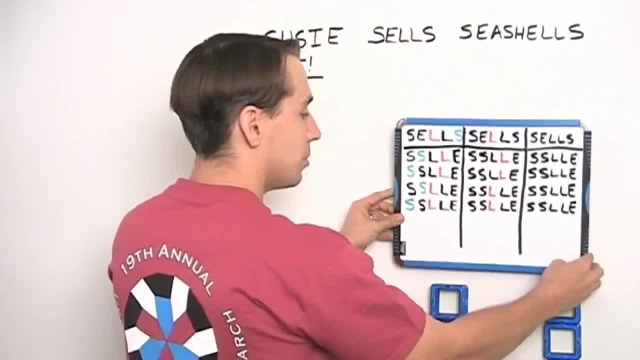 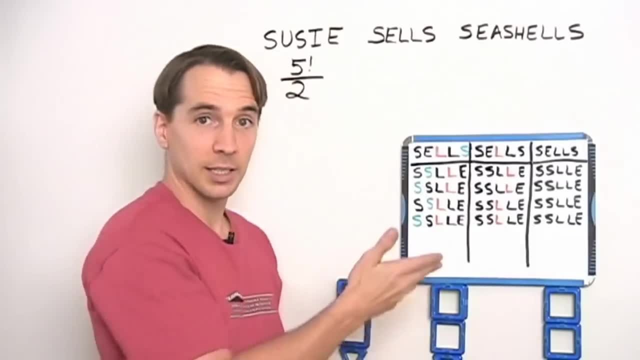 And this is where the magic time-saving device comes into play. There you go. I just saved you about five or ten minutes. Didn't save me five or ten minutes because I still had to write this whole thing, but you didn't either. 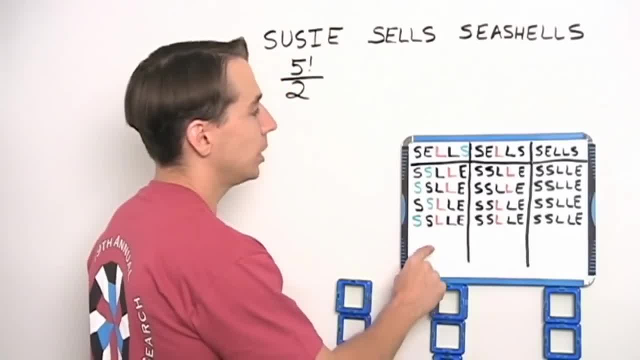 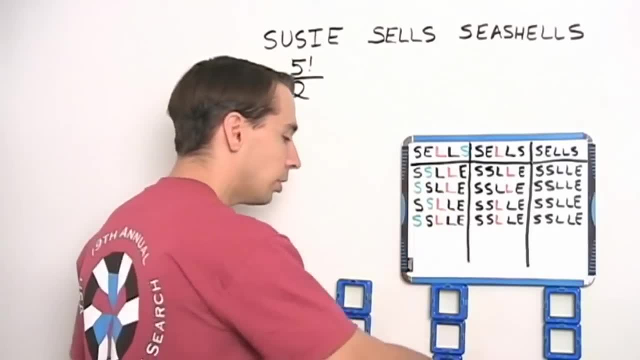 But you didn't have to watch me do it On our first column. here we're pretending our L's are different and our S's are different. Two different colors for the L's, two different colors for the S's. And we know that there will be five factorial words when we make that whole list. 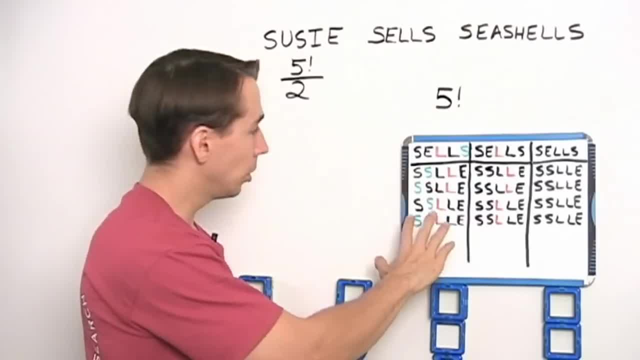 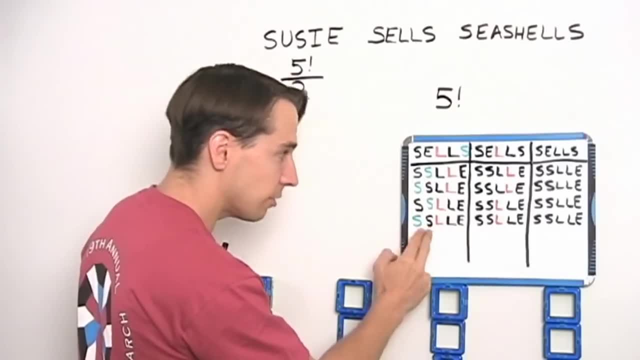 And then look at these four words here that we make. These are all different, All different, when the S's are different and the L's are different, And they all say S-S-L-L-E, but the S's are different, the L's are different. 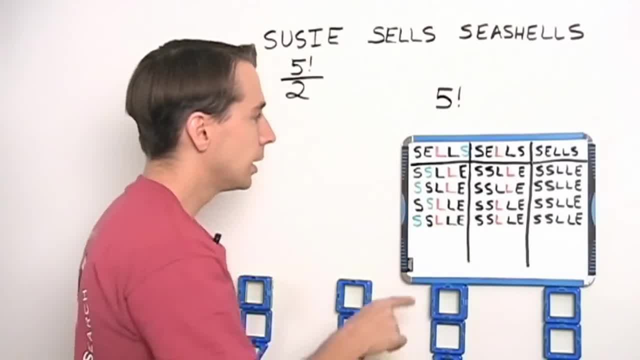 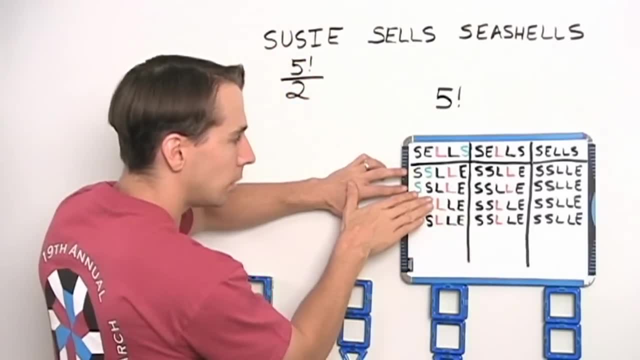 If you look at these four, four different words. Now look what happens when we make the S's the same. So look first at these first two words. When we make the S's the same, the only difference in these first two words is the order of the S's. 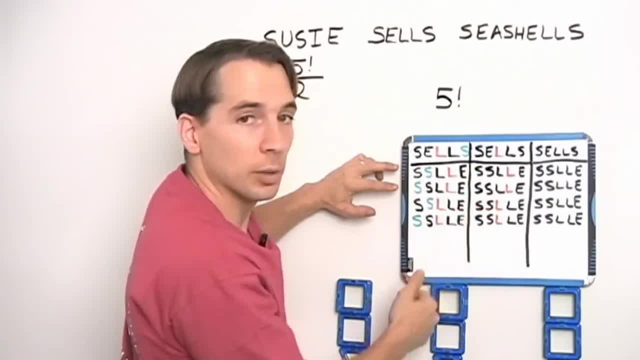 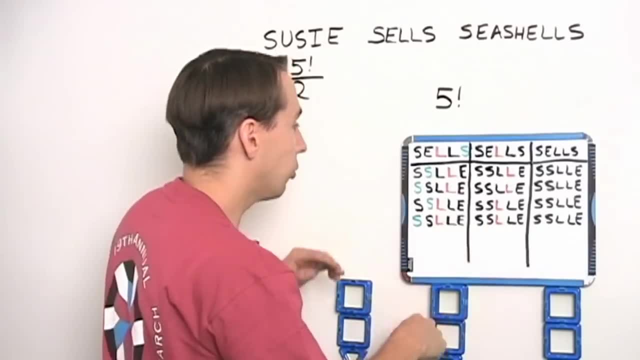 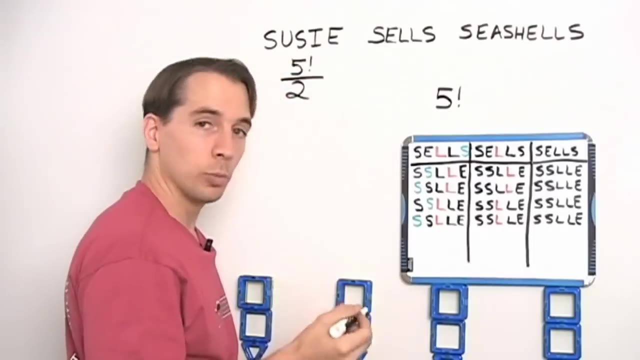 We make the S's the same, these two words become the same. Same thing down here: Make the S's the same, everything else is the same, so these two words become the same. So all the words in this list, all the words in this list, can be grouped into pairs, just like we did here. 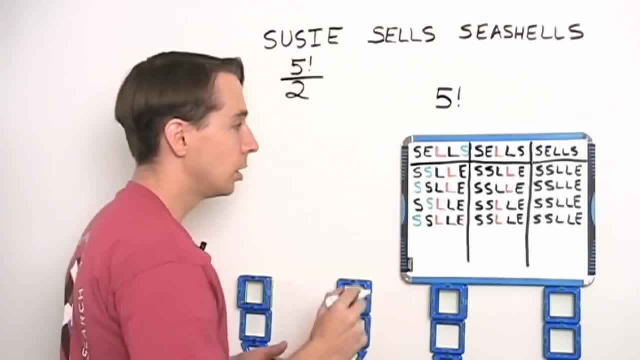 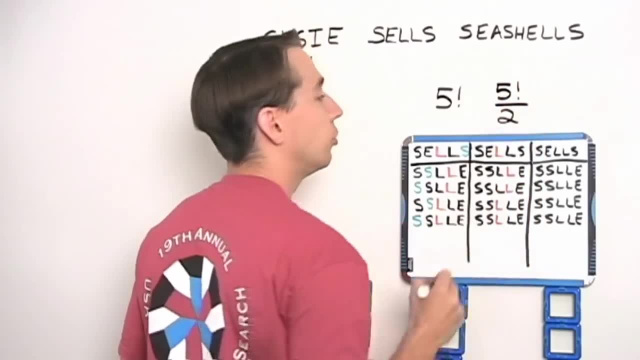 where in each pair the only difference is the order of the S's. So when the L's are different but the S's are the same, we have five factorial divided by two words. It's basically what we did over here with Susie. 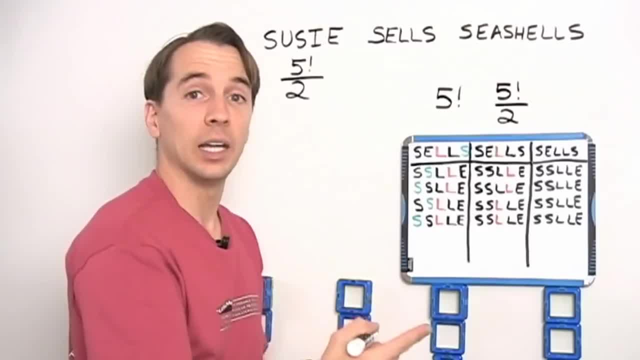 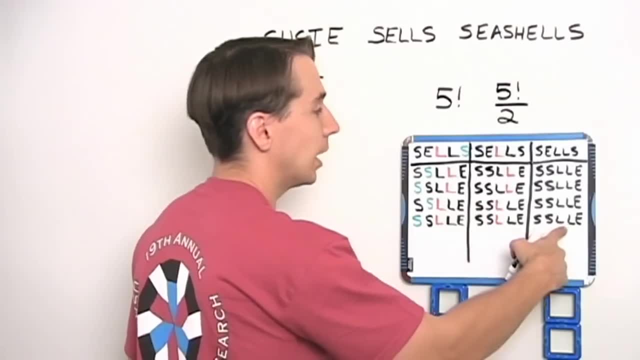 And then, when we go from this list onto this list, we see that we have to divide by two again for the L's. Here we have only two different words. And then, when we go onto the next step, well, now we only have one. 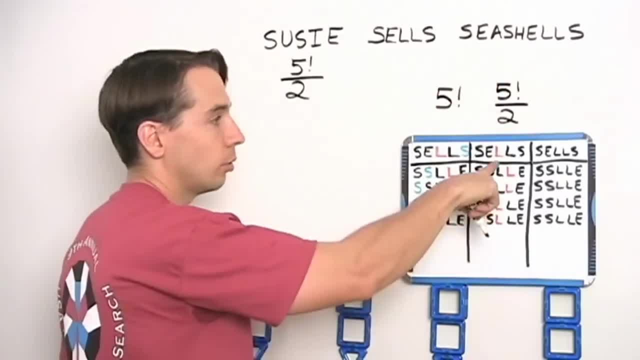 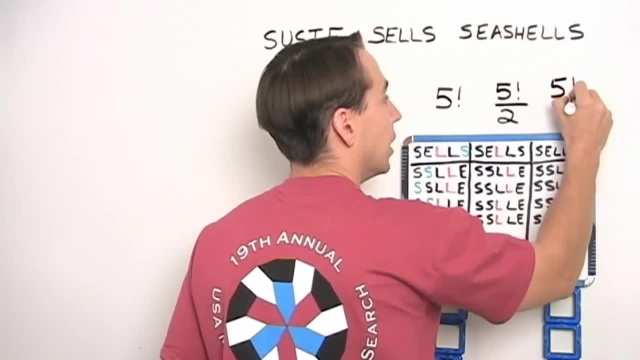 So when we take all the sixty, the five factorial, divided by two words, when the L's are different but the S's are the same, we can group them in pairs where the only difference is the order of the L's. So we're just dividing by two a second time. 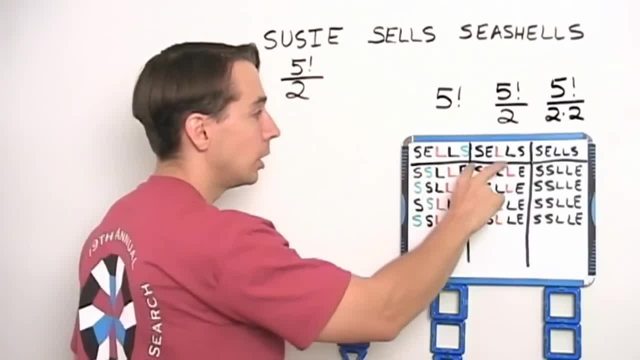 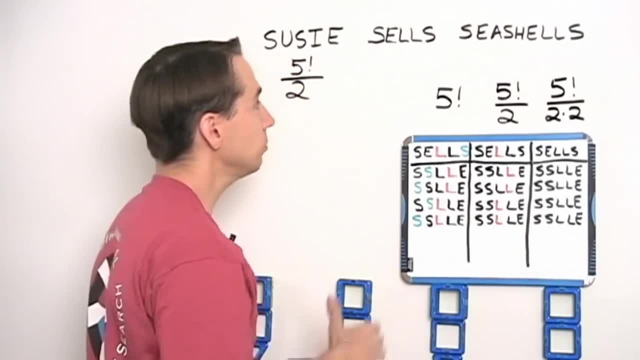 So again, we just start with our five factorial. All the letters are different. We divided by two when we made the S's the same, and we divided by two again when we made the L's the same. So we've taken care of cells. 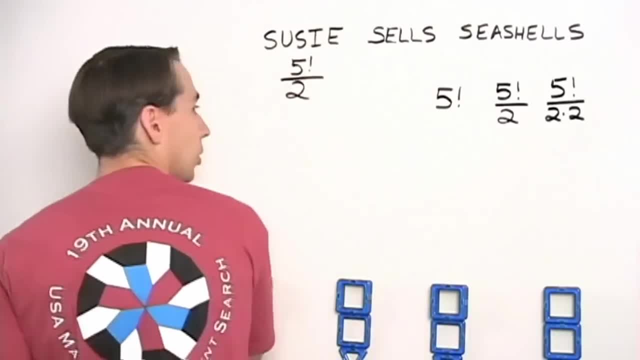 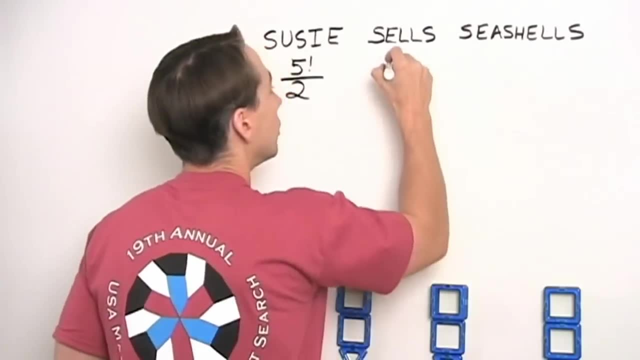 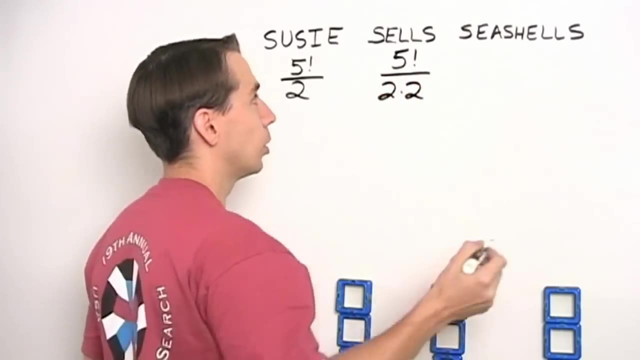 Don't need this anymore And we can go ahead and erase this. Write down our answer and move onto seashells. Now for seashells, we're all pretty confident where we're going to start. We're going to start with nine factorial because there are nine letters. 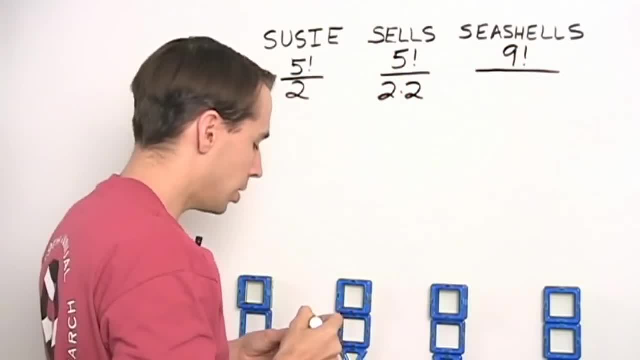 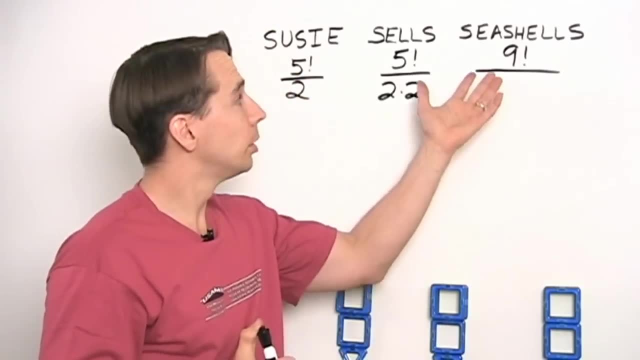 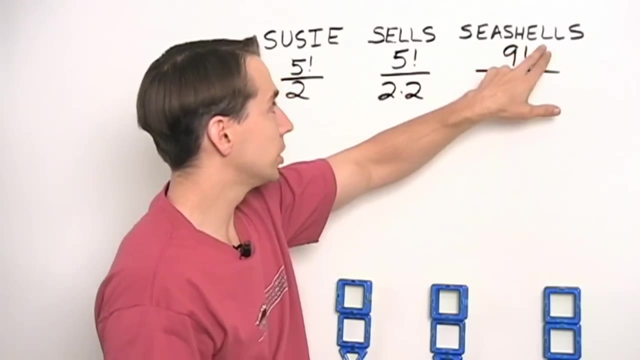 And we know we're going to divide by something. We're not sure what. What we want to divide by is the number of ways each word comes up in this nine factorial count. So if we just say we pretend the E's are different colors, 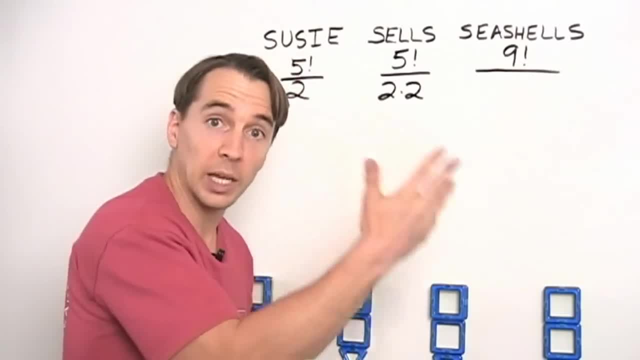 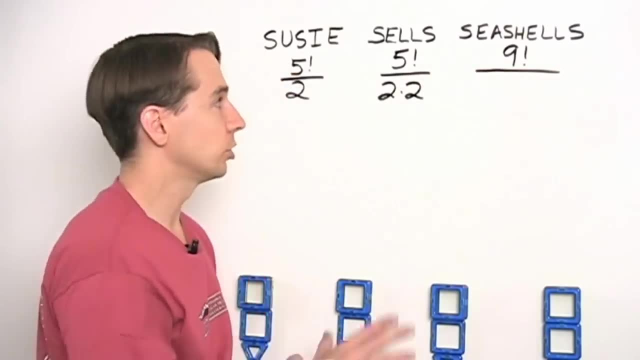 the L's are different colors and all three S's are different colors. well then, we would get nine factorial different words. But the word seashells is going to come up a bunch of times in there, just with the E's. you know, the coloring switch, the L's, the coloring switch or the S's. 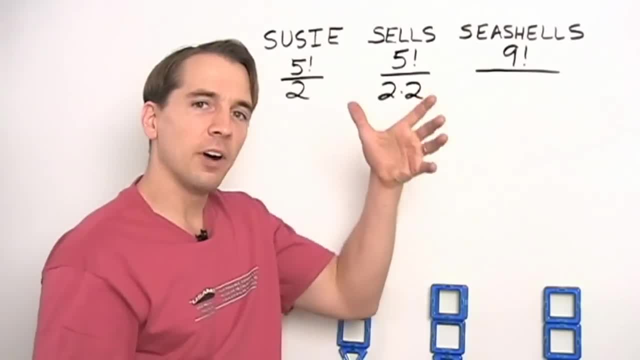 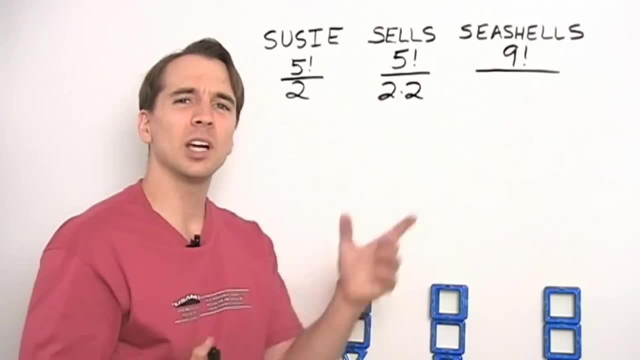 the coloring in a different order. So we have to divide by the number of ways we can produce each word the number of times each word comes up in this nine factorial list. But how many times do seashells come up if all of these are different colors? 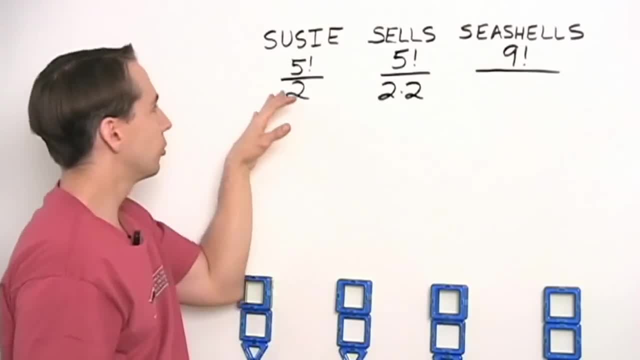 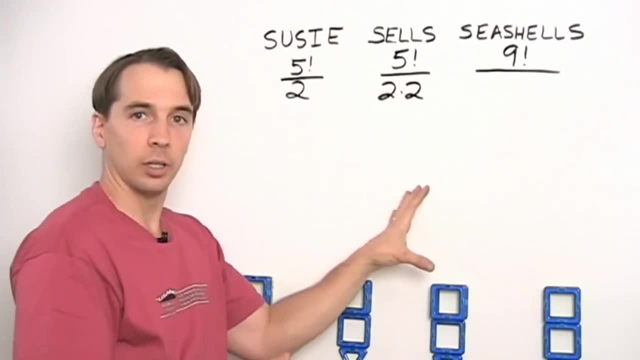 Well, we have a clue back here from these. For Susie, when we started with five factorial, each word came up twice. For cells, we found that each word. we saw that in the panel there we saw that each word comes up two times, two times when we start with five factorial. 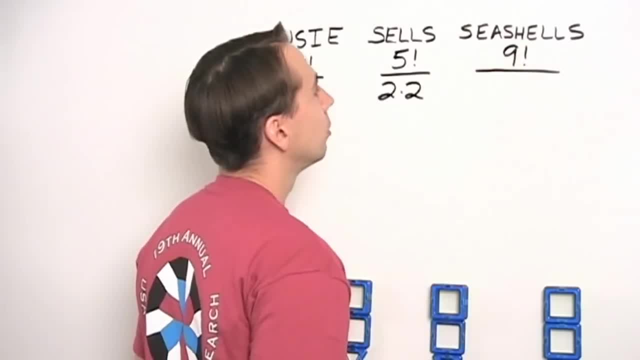 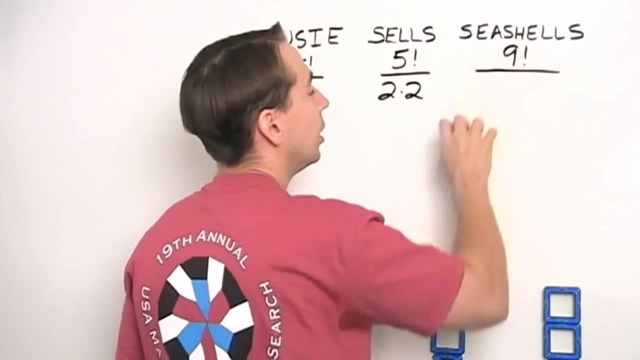 So what happens over here? Well, we have two E's. So if we were to take seashells here and color it, color the two E's different colors, two L's different colors and three S's different colors. well, how many ways can we choose our colors for the E's? 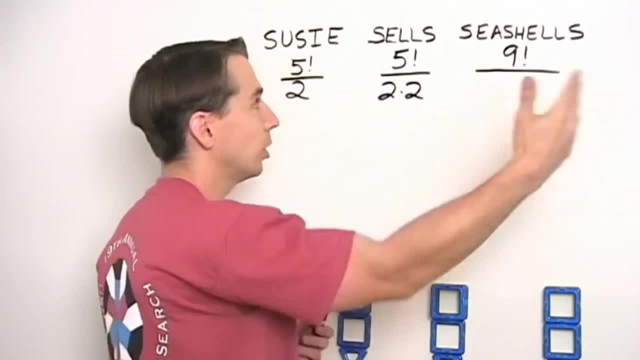 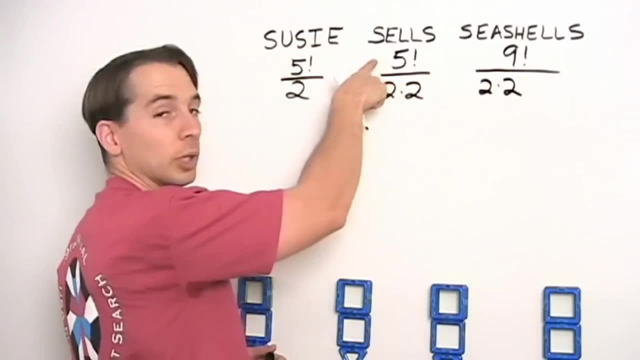 Well, there are just two. You have two colors to choose. for the first one, and then we use the other color on the other E, And then same thing for the L's, and it's the same thing we did over here. but what about the S's? 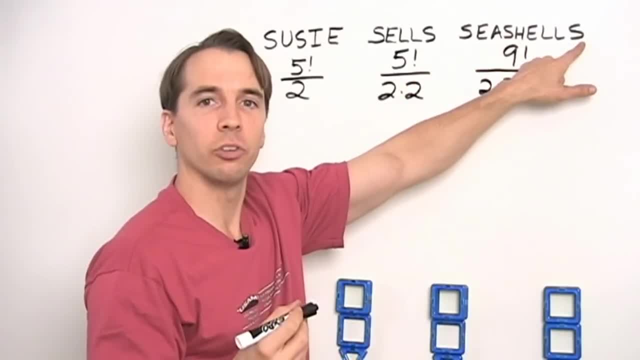 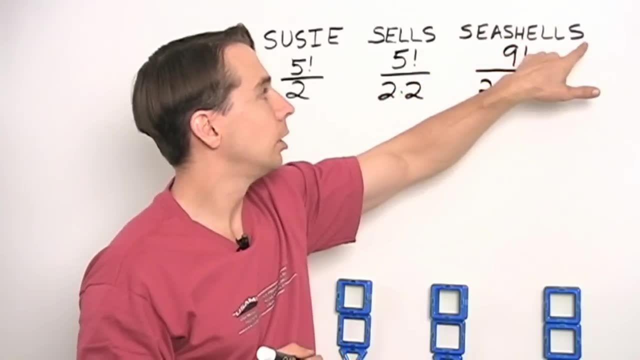 You know ways can I color these three S's with our three different colors? Well, we have three choices for the first color, two for the second and one for the last color. So there are three factorial ways I can color the S's. So instead, 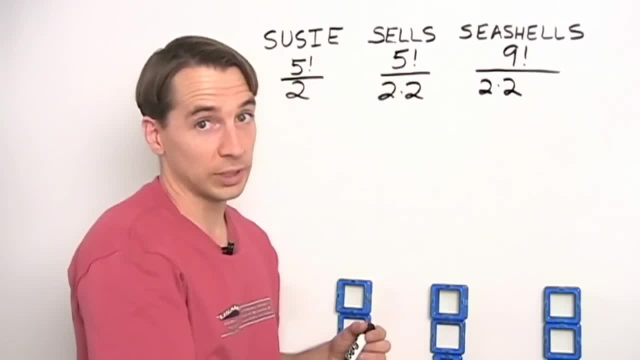 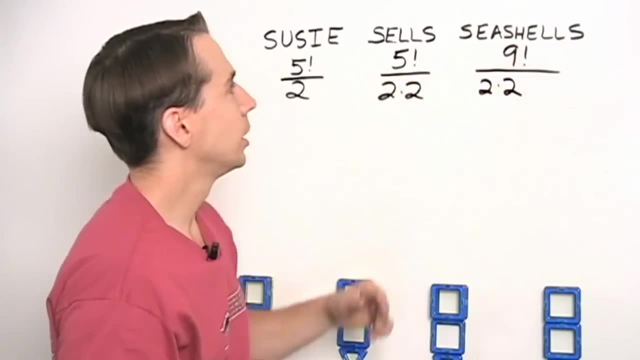 of thinking of it as listing out all the nine factorial words, which we're definitely not going to do, and then counting up how many times seashells comes up. we can instead think of it as: let's just start with this word and see how many ways we can. 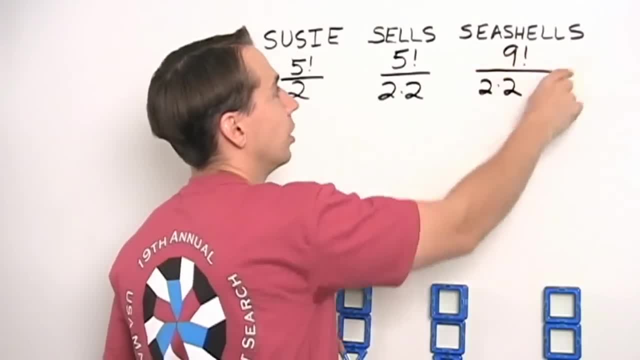 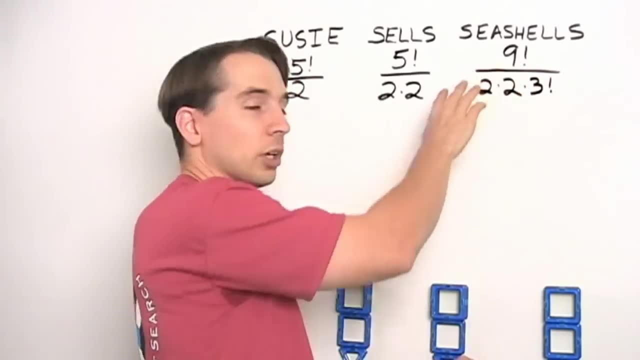 color it. E's two different colors, L's two different colors and then S's three different colors. And we see that there are two times, two times three factorial ways that we can color our E's, color our L's and color our S's. And that means that when we start with our nine factorial 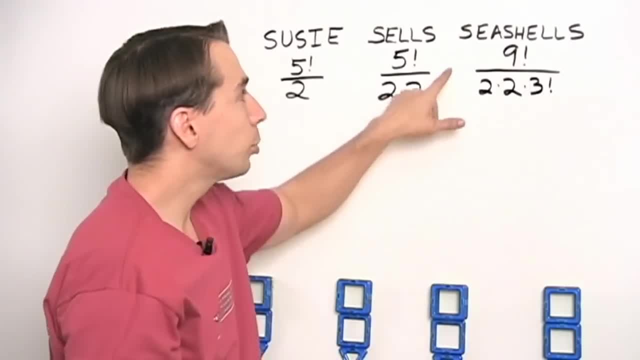 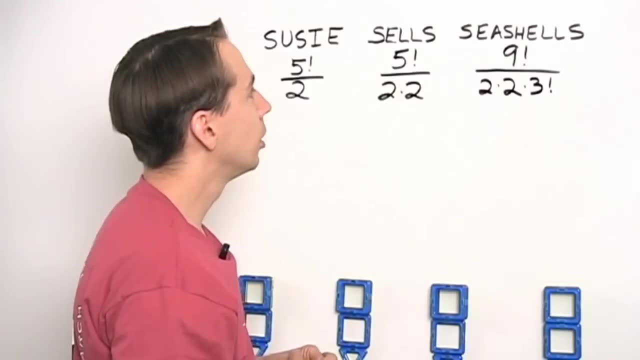 our list of nine factorial words, we'll produce the word seashells two times. two times three factorial times one for each, way that we can color those letters. You're not convinced, are you? I'm not entirely convinced either. It's kind of wordy and it's much. 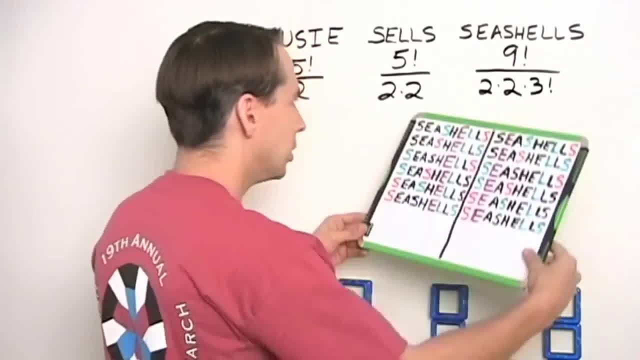 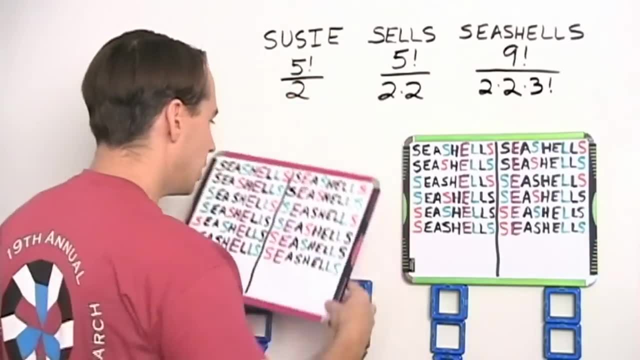 better to take a look at an example and then we'll come back to our explanation and see if it's more convincing. What we did here is: I took seashells and you can see I've colored the E's two different colors: purple and black. 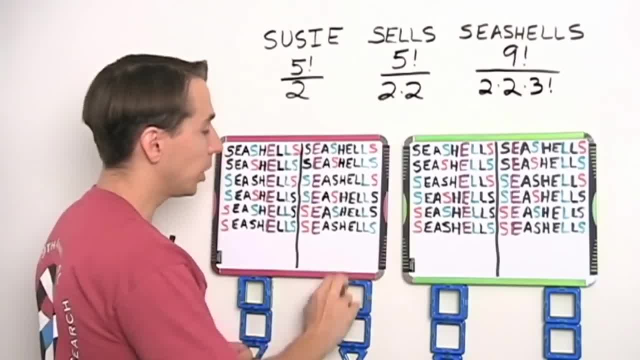 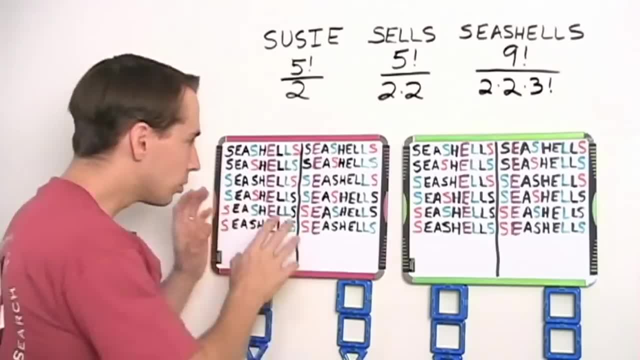 colored the L's two different colors- green and black- and I've colored the S's three different colors- green, black and red- And the first thing I did is I grouped them up here- magical time-saving devices. you certainly didn't want to watch me write this. 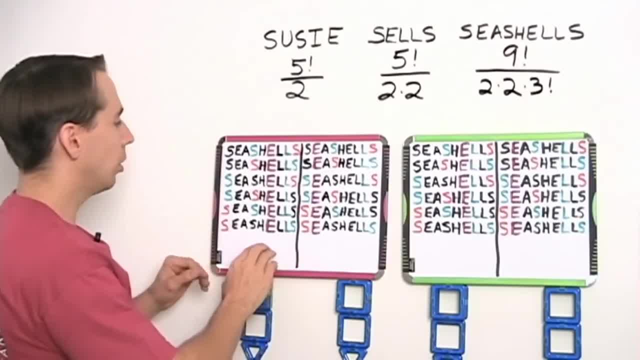 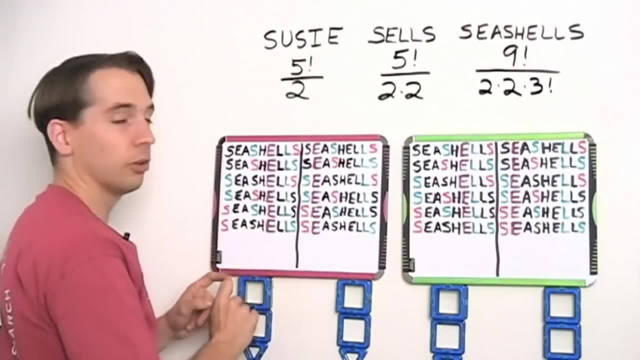 I grouped them by how the E's and L's are colored. So here all the E's, the first one's black, the second one's purple. First L is black, second L is green. And then here: first E is purple, second E is black. first L is black. 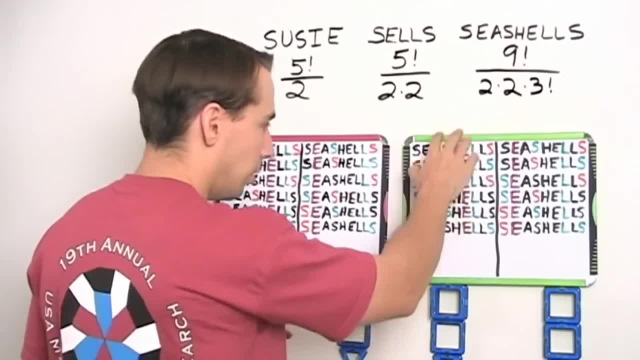 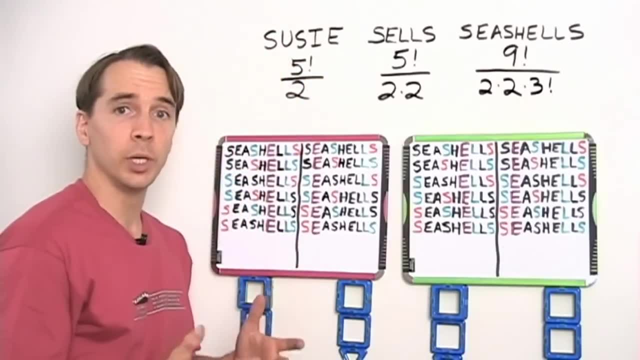 second, L is green, And here all of them in this column are the same. all of them in this column are the same, just the E's and the L's. And we know that there are two times two, just four ways to color the E's and the L's. You know two times two ways we can do this are: 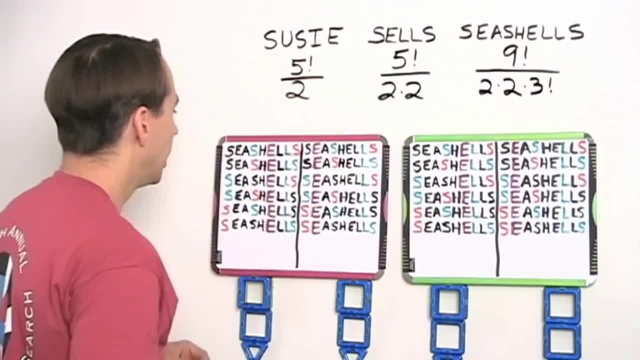 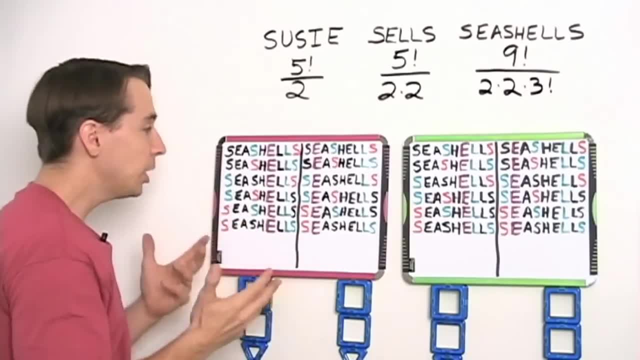 two for the E's, two for the L's. It's basically the same thing we did here, And then we look at each one Here. when we have the first E black, second E purple, first L black, second L green, how many ways can we color the S's? 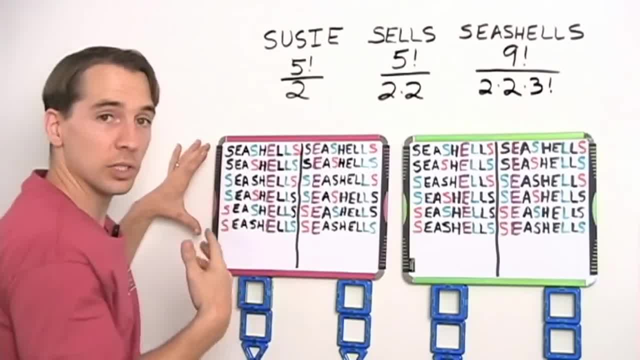 And we see there are six. We can see that in our list or we can just think it out. We're going to use a black and a green, A black, a red and a green. S Well, we have three choices. 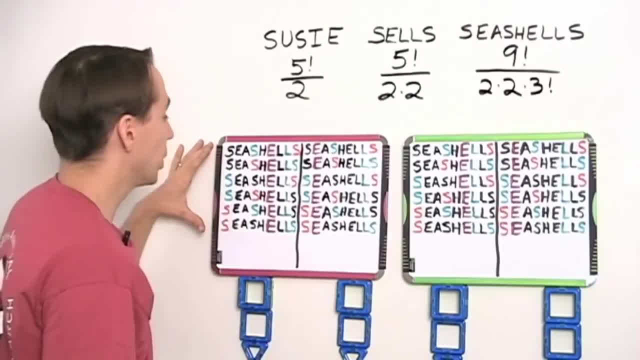 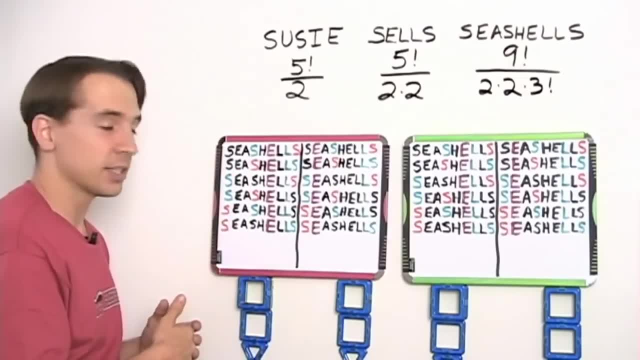 for which one comes first, two choices for which one comes second and one for which one comes last. So for each of these four ways we can color the E's and the L's. there are six ways to arrange the S's. So, sure enough, there are two times, two times three factorial ways. 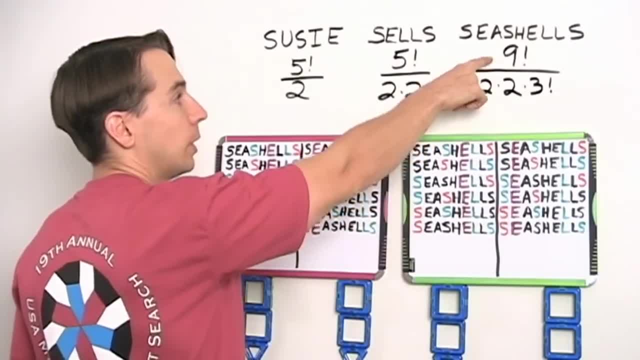 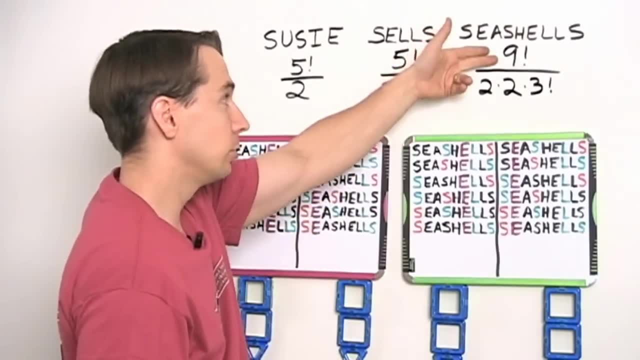 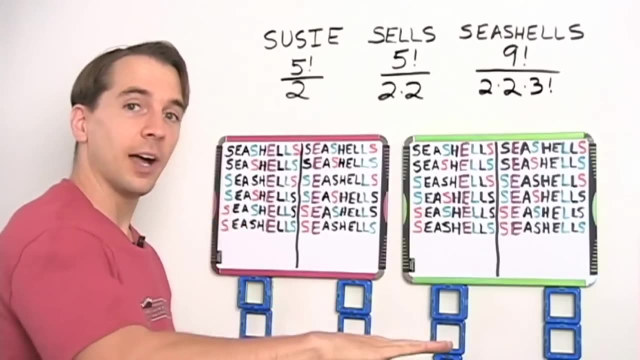 that we produce the word seashells when we write nine factorial, And the same is true for every single word that we produce. So when we start with nine factorial, we produce every single possible word two times, two times three factorial times. So we have to divide, to correct for that over counting. 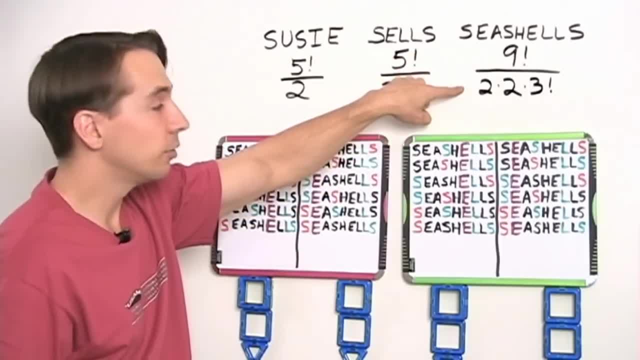 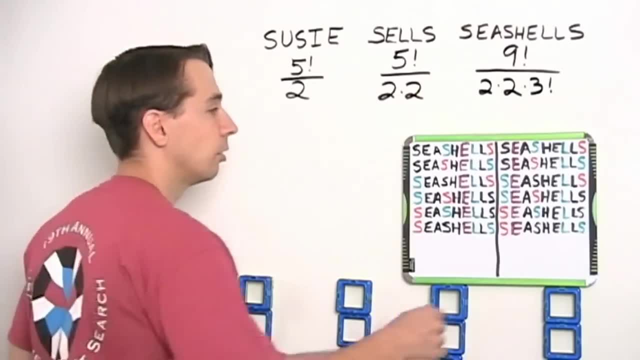 So the total number of different words we get is just nine factorial divided by two times two times three factorial. And now we're ready to go ahead and compute these. We'll get rid of this and get rid of this, And we have five factorial divided by two. 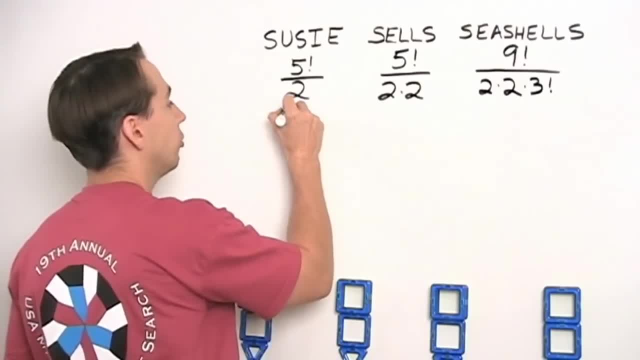 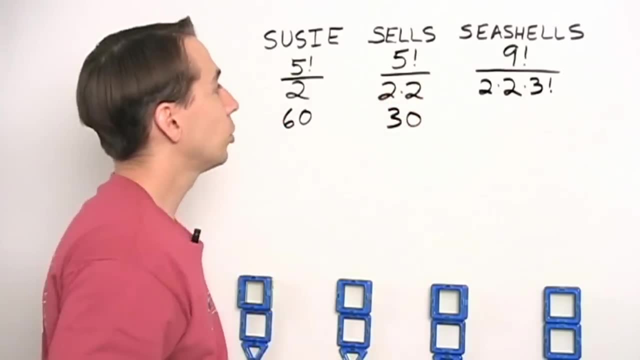 five factorial is a hundred and twenty divided by two is sixty, And then over here we divide it by two again, sixty divided by two is thirty, And then nine, factorial divided by two times two times three factorial is twenty-four. obviously, this is fifteen thousand one hundred and twenty. 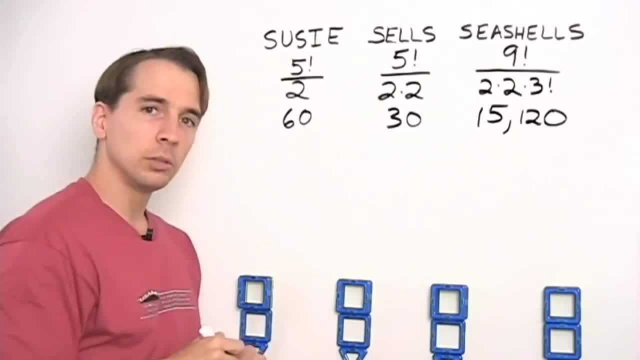 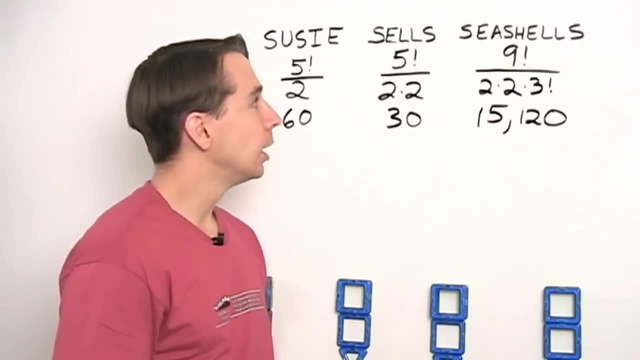 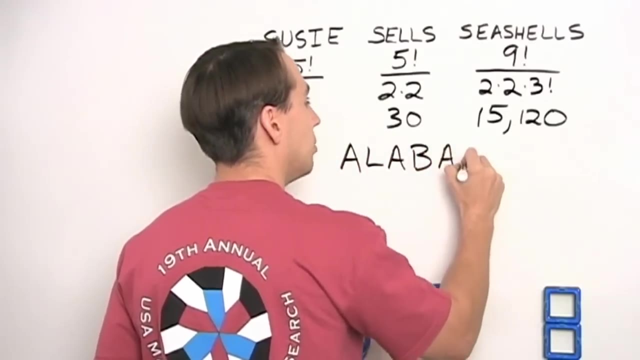 Moreover, you should now get an idea of how to handle any word. So you take any old word, you can write down, and I'm going to write down Alabama. I went to high school in Alabama And you can imagine how many math contests I went to that asked me how. 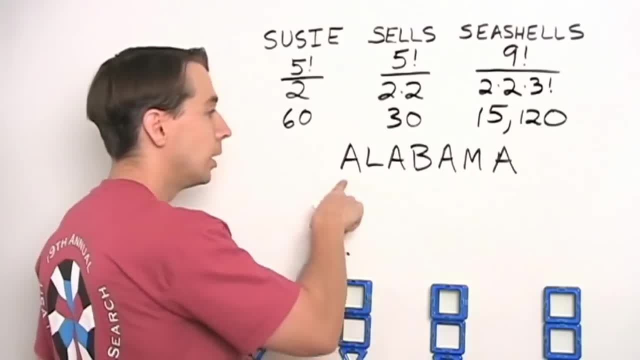 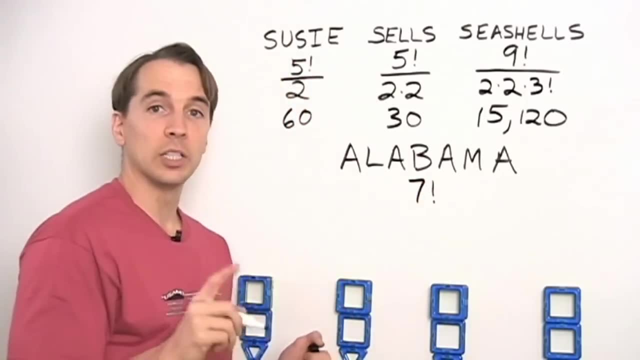 many words can be formed by arranging the letters in the word Alabama. So you take any old word, count the number of letters. we have seven letters, So there are seven factorial arrangements. However, we have to divide to correct for over counting if we have any repeated letters. 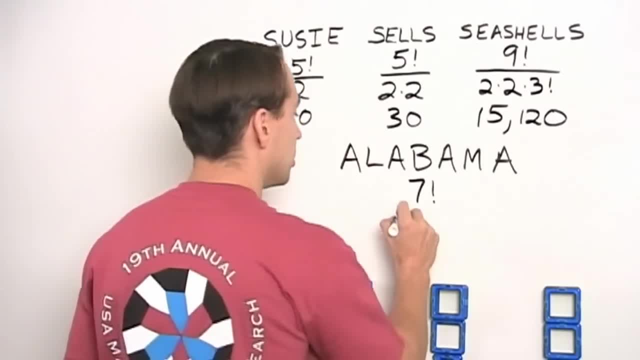 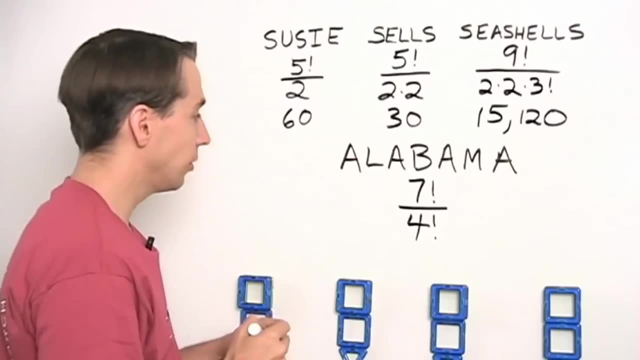 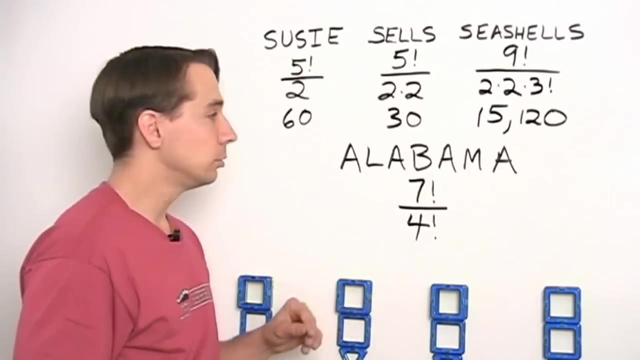 Four A's. there are four factorial ways to arrange the A's, So each word in our seven factorial count will be produced four factorial times. It's just seven factorial divided by four factorial. You can figure that one out in your head right. So now you know how to handle any word.